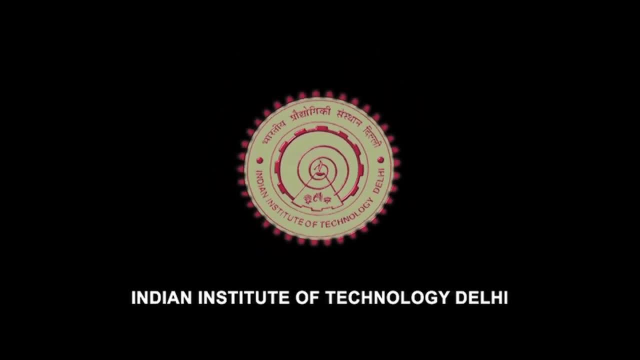 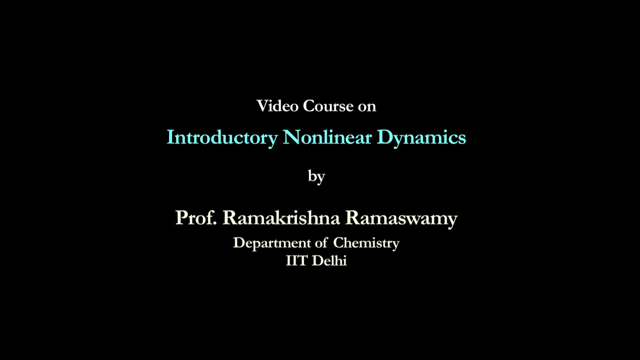 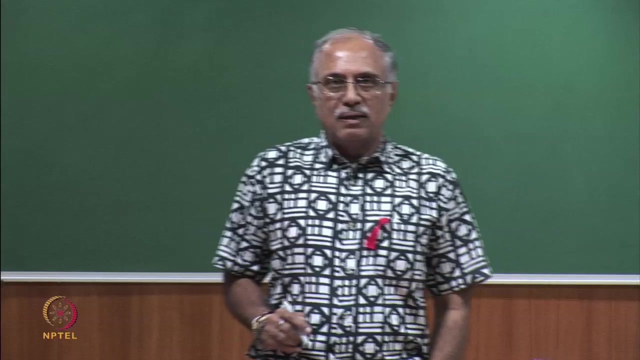 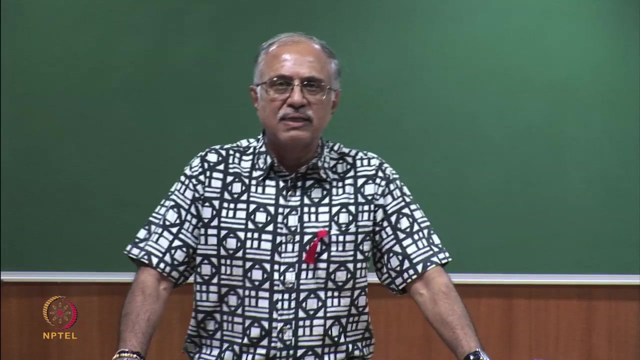 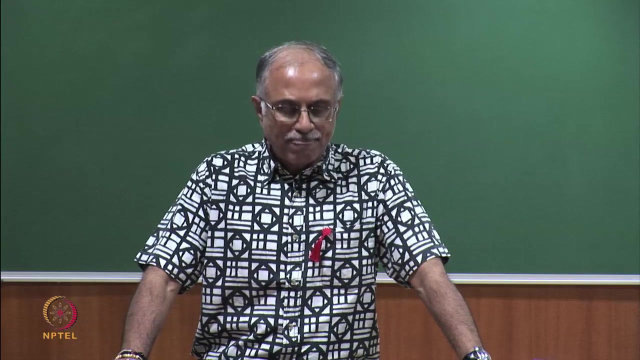 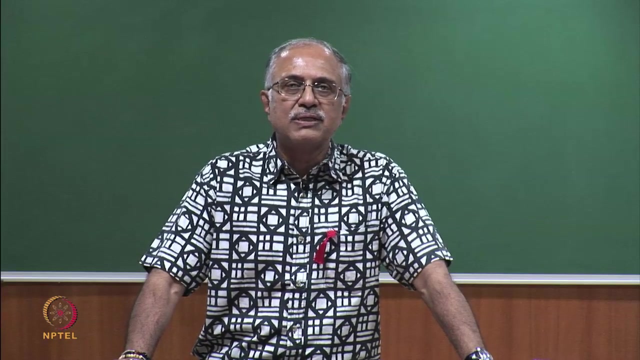 Hello, this week we are going to be looking at Characterizing Chaos and as a first step I would like to discuss fractals today. Recall that in the last lecture we were looking at the bifurcation diagram for the logistic map and towards the end I pointed out one curious. 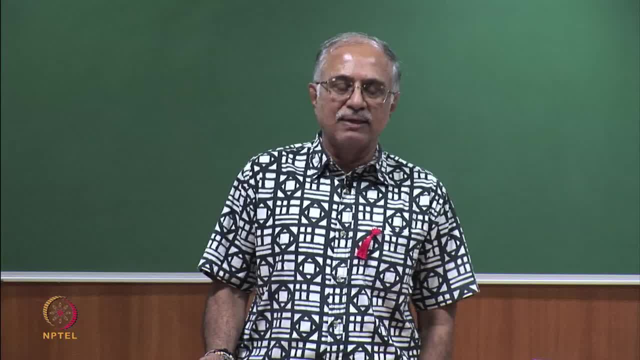 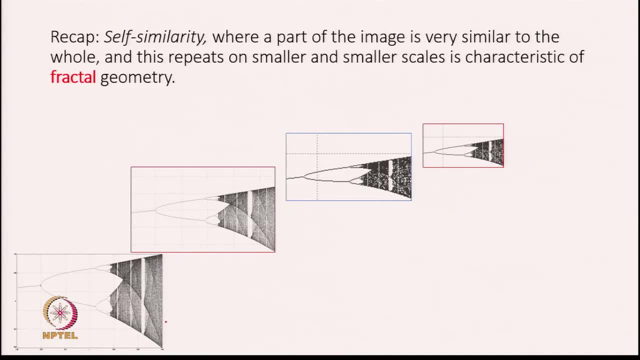 feature of this bifurcation diagram, namely that when you consider the whole bifurcation diagram which is shown here in the extreme left of your screen, Then a small part of the bifurcation diagram, when expanded, looked pretty much like the original diagram itself, and when you took a small part of that and expanded it it looked 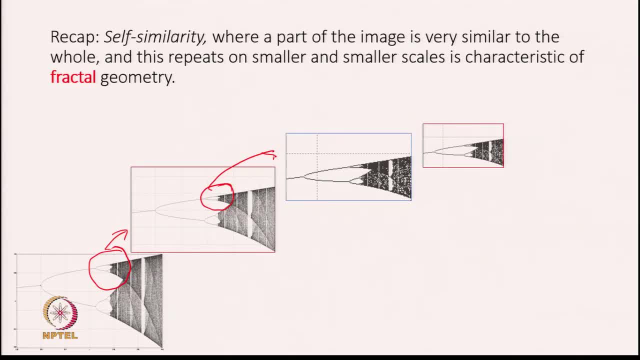 pretty much like the whole bifurcation diagram itself. So you can take a small part of that and expand it, and so on, and so on ad infinitum. This kind of geometry is described these days by what is termed fractals, and the fact that 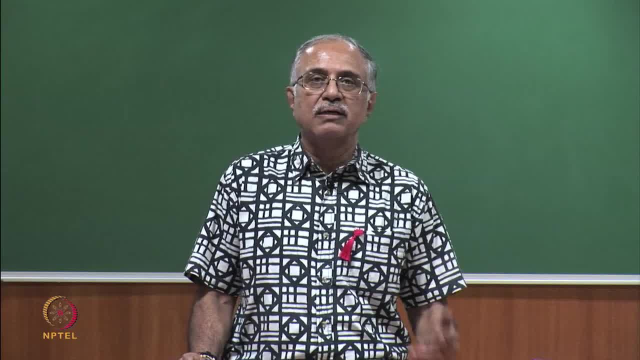 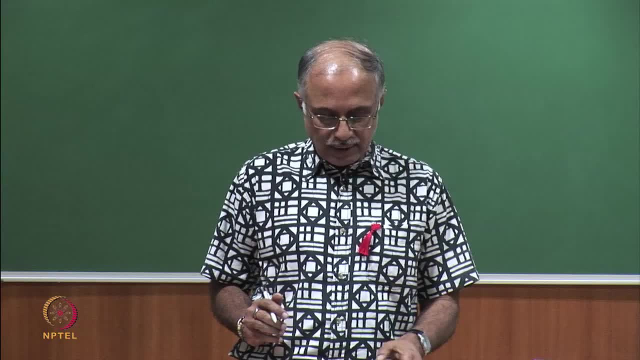 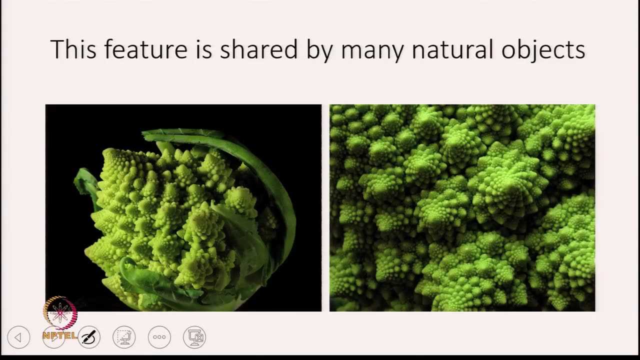 a certain structure in the object occurs on smaller and smaller scales is characteristic of fractal geometry. The architects also share this feature. Spectacular example is that of a head of Chinese broccoli. When you look at the broccoli head, you can notice that it is consisting of many little 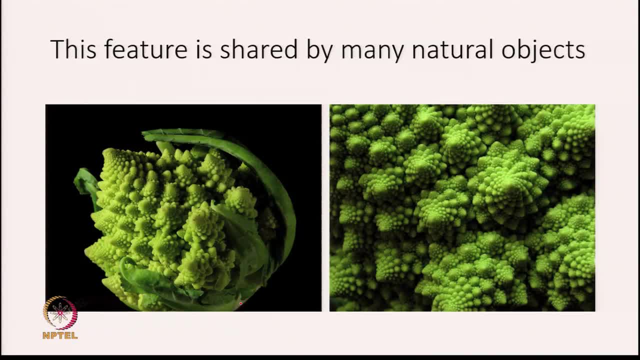 module nodules over here and when you expand it you can see that the structure of each of these nodules is extremely intricate. But if you focus on one of them, you can see that each of these looks pretty much like the whole nodule itself and the whole structure is repeated. 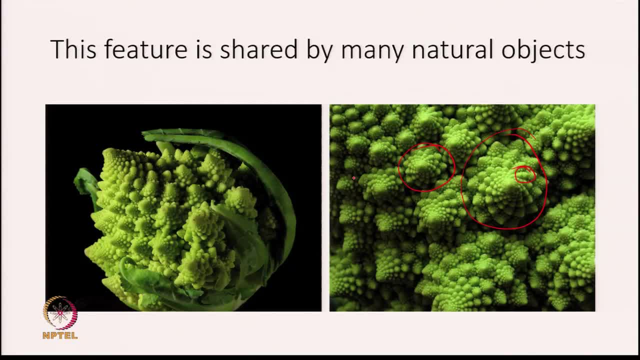 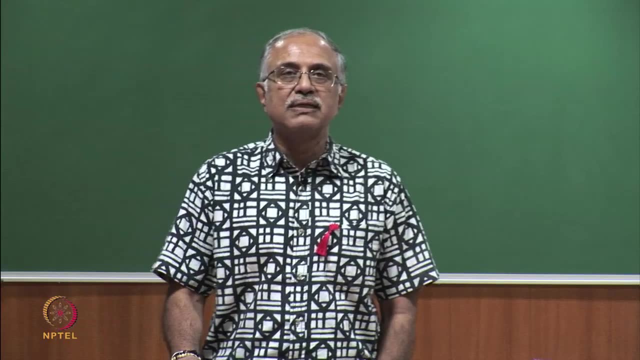 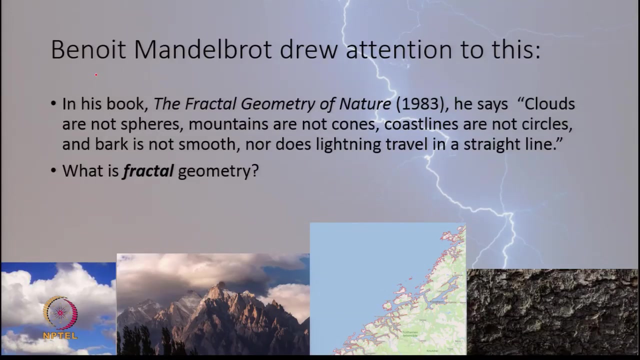 endlessly in this, in this broccoling. Many natural objects have this feature, if not precisely statistically, they have this kind of feature, and the first person to draw our attention collectively to this is a mathematician, Benoit Mandelbrot, who from the 50s onwards was pointing 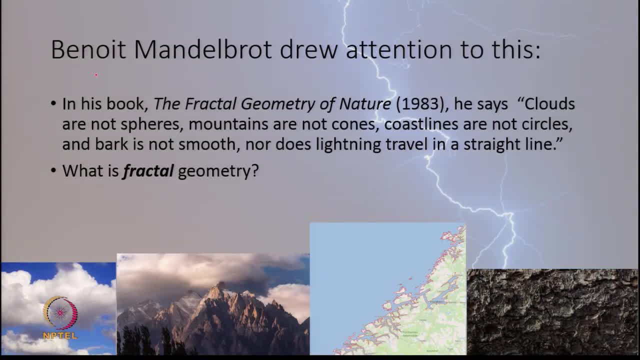 out that standard geometry is not enough to describe a whole variety of natural objects. In his very influential book the Fractal Geometry of Nature in 1983, he says: clouds are not spheres, mountains are not cores, Coastlines are not circles and bark is not smooth. nor does lightning travel in a straight. 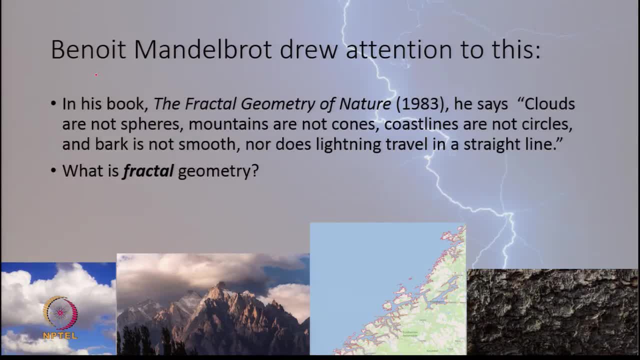 line. He was drawing attention to the fact that when modeling something like a cloud to a first approximation, a cloud is like a sphere, But, as you can see, this cloud is far from spherical and even the sphere has little features on it On smaller and smaller scales. A first approximation to a mountain might be a cone, but this mountain 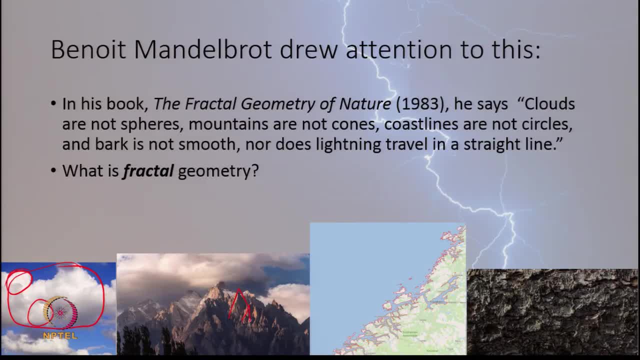 as you can see, has structure. there are other mountain, the other little cones on top of cones, and so on and so forth. So if you really wanted to describe what a mountain look like, it would not be by a simple cone Coastline, The coastline of 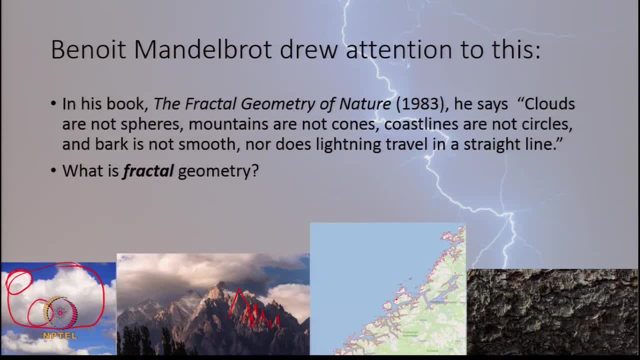 Of a country or the border of any particular country is not always very smooth and, in particular, a coastline cannot be approximated by a circle. The bark of a tree is not smooth. it is not a, it is not some smooth surface, but it has a lot of structure on it, as you can see in.